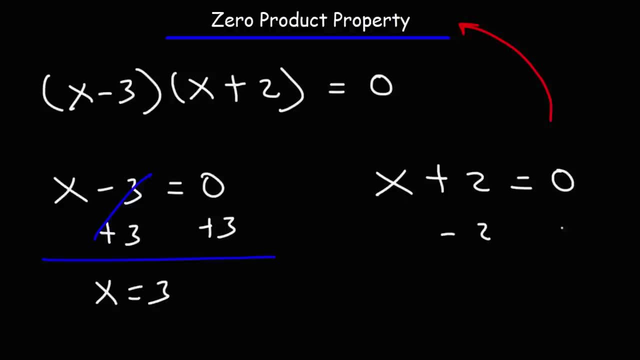 And we'll get x is equal to positive 3.. For the second one, we need to subtract both sides by 2. And we'll get x is equal to negative 2.. So that's one of the applications of using the zero product property. 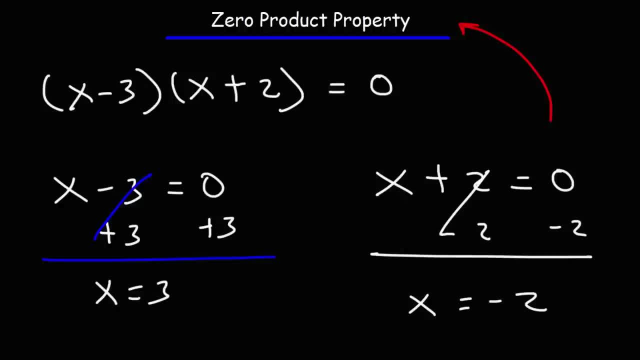 It's very useful when solving quadratic equations, especially when you're factoring. For the sake of practice, go ahead and calculate the value of x for these two equations. The first one is going to be 3x times x minus 7 is equal to zero. 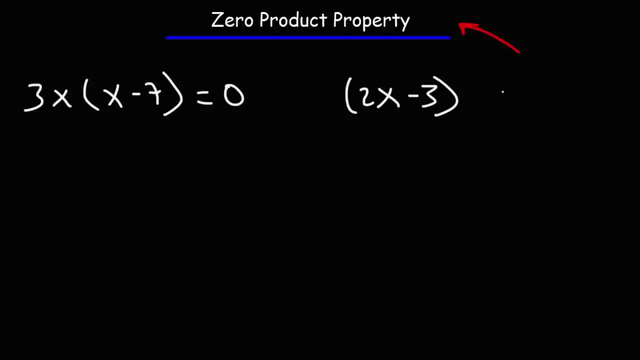 And for the second one, it's going to be: 3x times x minus 7 is equal to zero. And for the third one, it's going to be 2x minus 3 times 3x minus 5 is equal to zero. 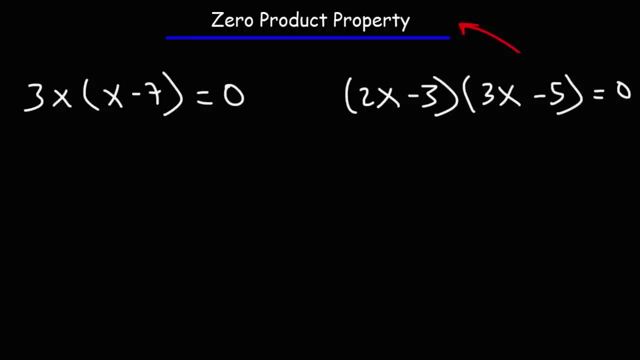 So use the zero product property to calculate the value of x for each of these two equations. Now for the first one, what we can do is we can set each factor equal to zero. So we can set 3x equal to zero and x minus 7 equal to zero. 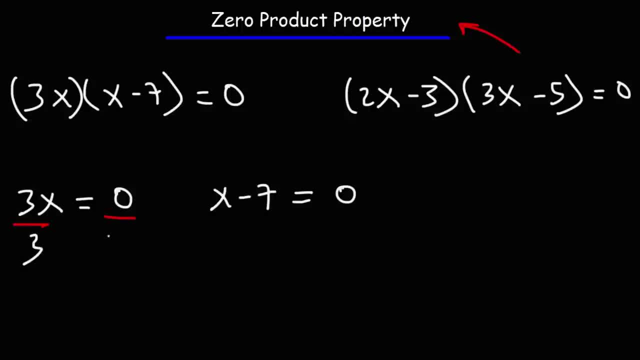 For the first one, we need to divide both sides by 3.. 3x divided by 3 is simply x. Zero divided by 3 is zero. So the first answer is just: x is equal to zero. For the second equation, we simply need to add 7 to both sides. 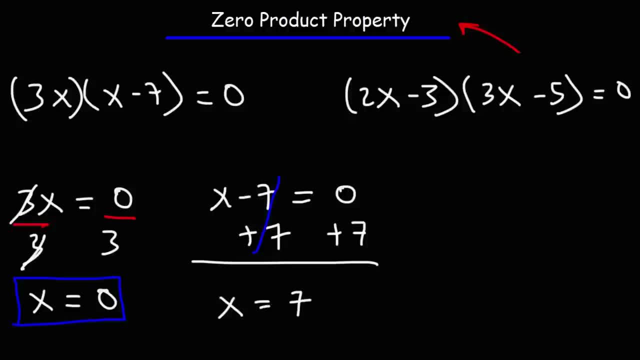 And we get the answer: x is equal to 7.. So if we were to plug in zero or 7 into the original equation, it's going to work. For instance, if we plug in zero into each x value, we'll have 3 times zero, times zero minus 7.. 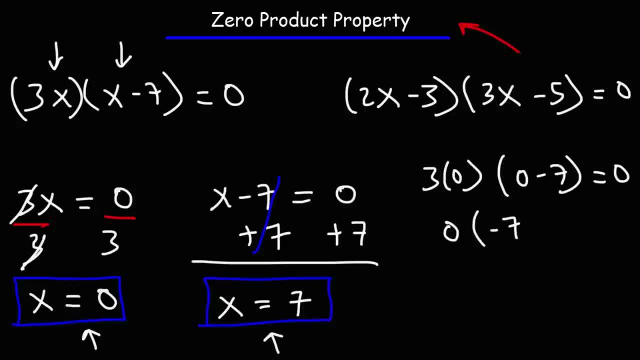 3 times zero is zero. Zero minus 7 is negative 7.. Zero times negative 7 is zero. So this works Now if we plug in 7, it will work as well: 3 times 7 and then 7 minus 7.. 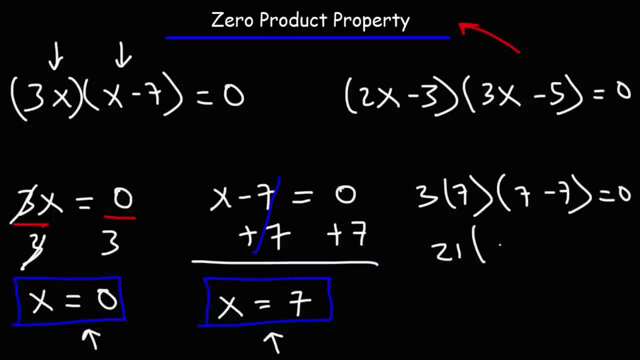 That's going to be zero. 3 times 7 is 21.. 7 minus 7 is zero. 21 times zero is zero. So using the zero product property, we can solve for x whenever it's in factored form.